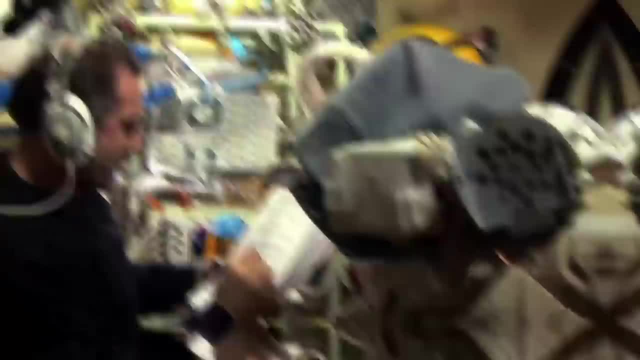 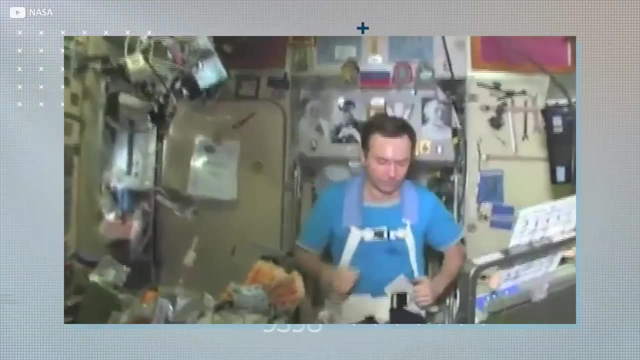 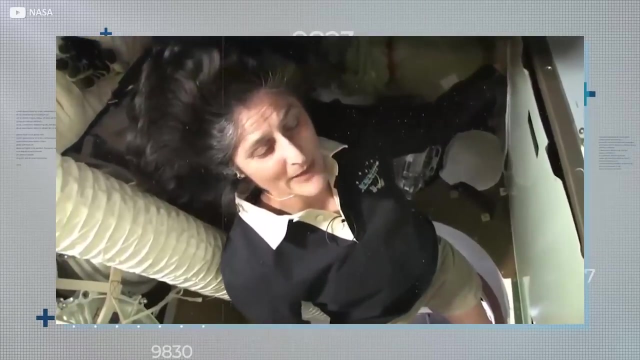 or check any overnight missions sent across from mission control. First things first, a hop in the shower, right? Well, no Astronauts can hope for hygiene-wise, despite working out twice a day- is to squirt a pouch of warm water and a trace of soap onto a washcloth to rub themselves down with Longer-haired crewmates. 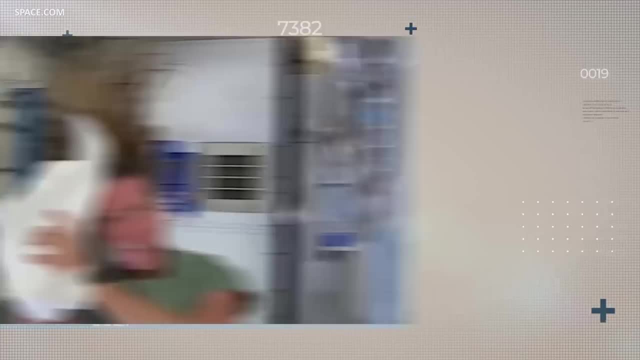 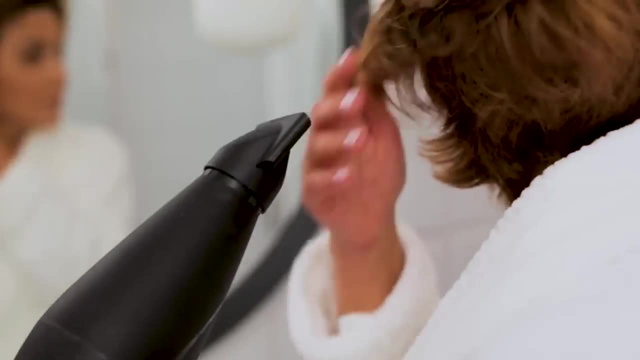 like to use a special rinseless shampoo applied to their scalp and rubbed vigorously through with a towel. This requires very little water and was developed for hospital patients who can't shower. At least you never need a hairdryer. There's even a specially adapted hair-cutting machine. 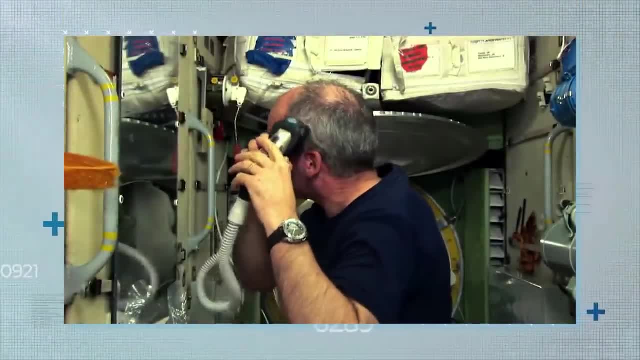 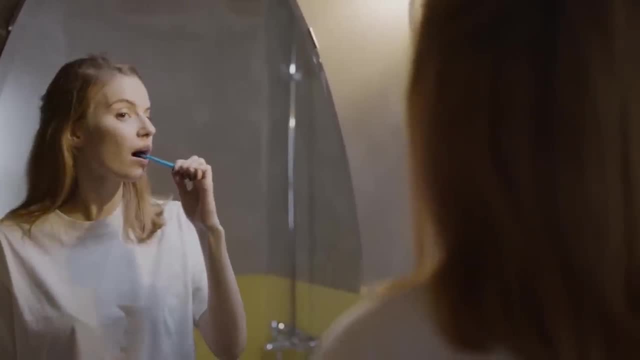 called the Flowbee, Essentially a pair of clippers attached to a vacuum cleaner which prevents stray stubble from floating, causing the hair to fall away and clogging up vital ISS hardware. Toothbrushing is broadly similar to the process on Earth and astronauts are even allowed to bring 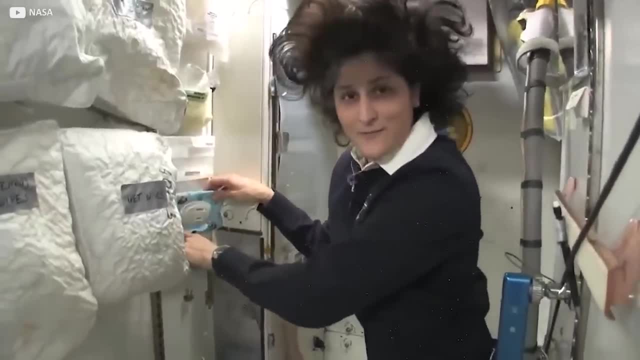 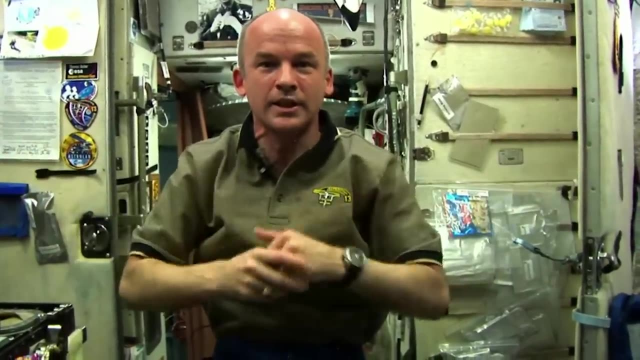 up their own preferred brand of toothpaste. The main drawback is, with no sinks or running water, astronauts pretty much have to swallow at the end. It's time to get dressed. Astronauts usually wear casual short-sleeved t-shirts as the temperature aboard remains. 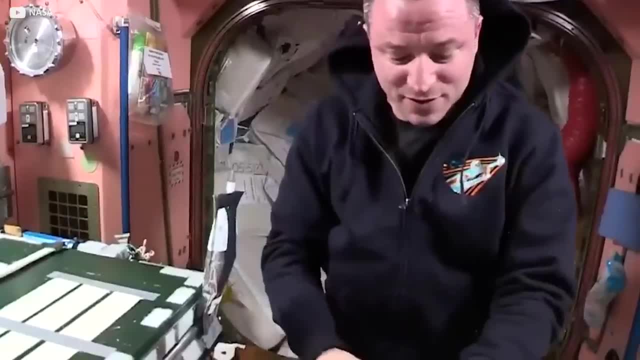 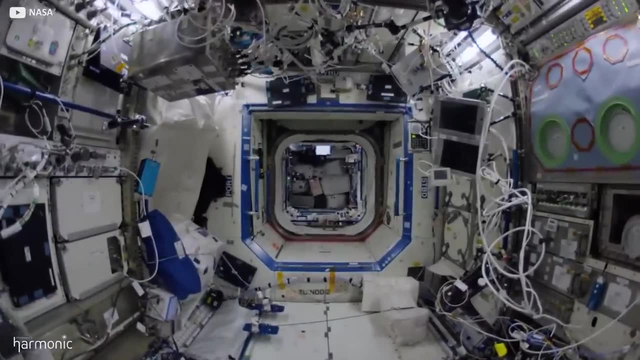 a constant 72 to 73 degrees, and there's rarely any reason to get dolled up or wear a jumper. They change their clothes as seldom as possible and they wear the same items for days at a time. This is because there isn't much storage space. 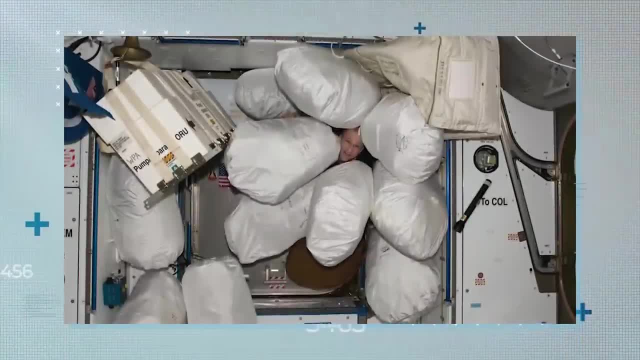 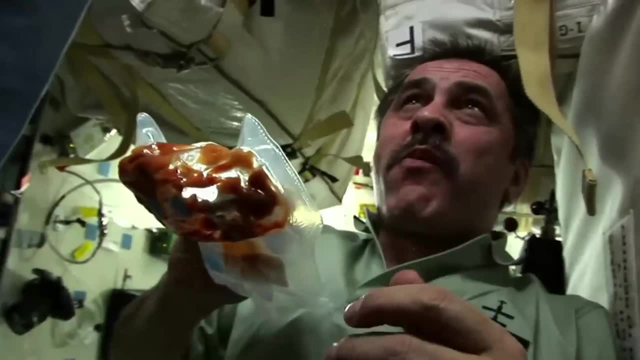 and certainly no washing facilities on the station. After a few days, the smellier items are stashed in a mesh bag, ready for the next resupply mission to dispatch to a spectacular fiery death on re-entry, hopefully having brought fresh supplies beforehand. 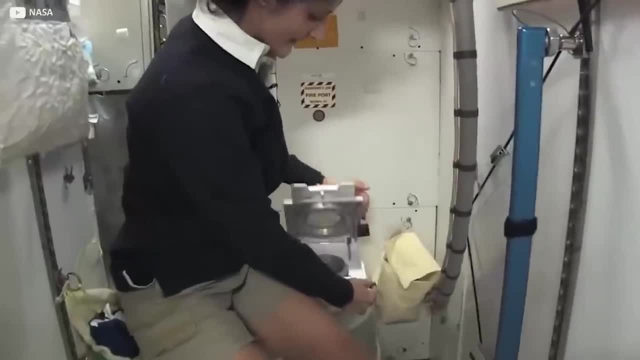 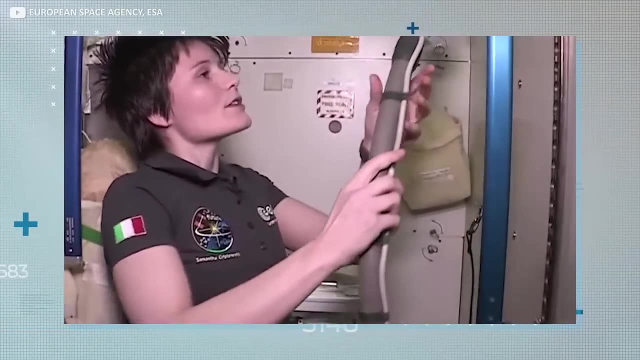 Inevitably, even in space, nature calls. As you might expect, visiting the bathroom in a microgravity environment throws up an assortment of grim challenges. For liquid waste, each crew has a personal urinal funnel they attach to a fan-driven vacuum hose. This fan sucks any and 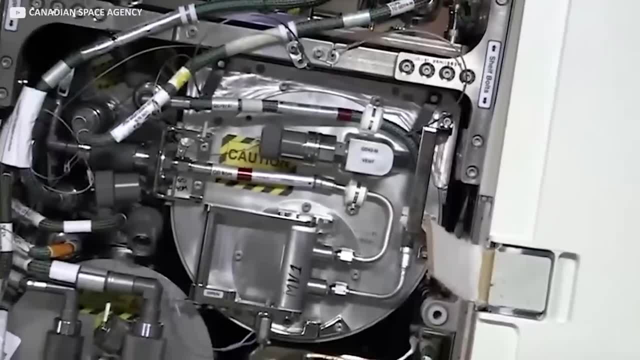 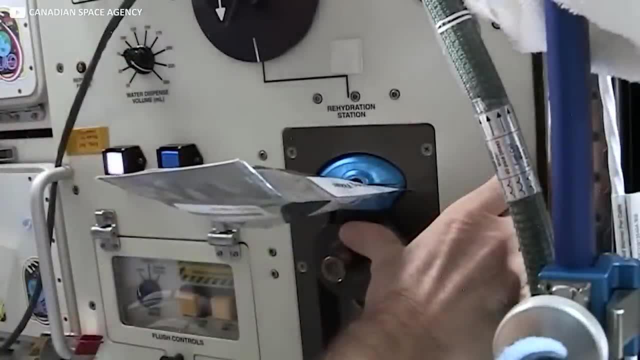 all liquids away, whisking just next door where, alongside moisture condensated from the air, their wee is broken down by electrolysis to generate fresh oxygen and make the next batch of drinking water. Solid waste has its own, wholly separate system. Well, it's the same fan. 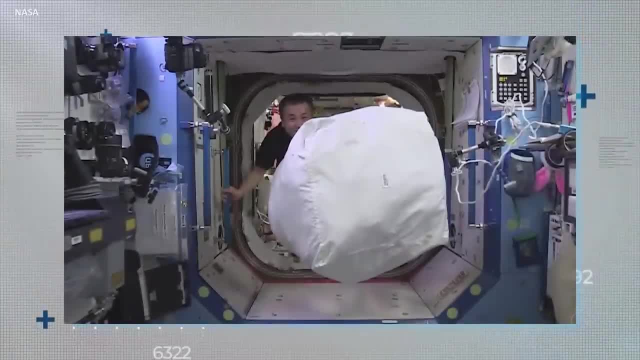 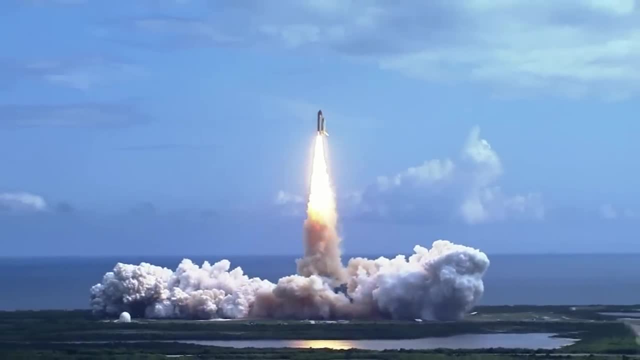 Feces are sucked away into a wastewater tank and sealed in a plastic bag. It's considered good etiquette, by the way, for astronauts to at least try and remember to leave a fresh bag for the next crew person. Unlovely as this setup is, it's a vast improvement on 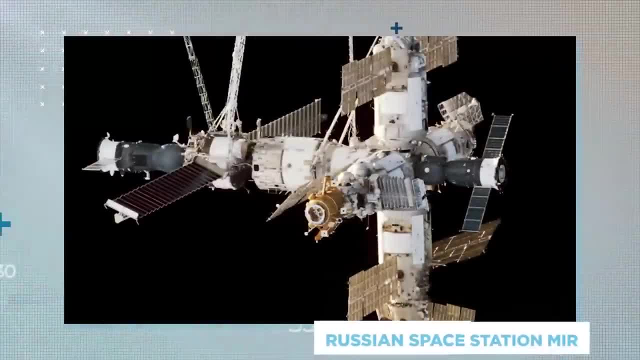 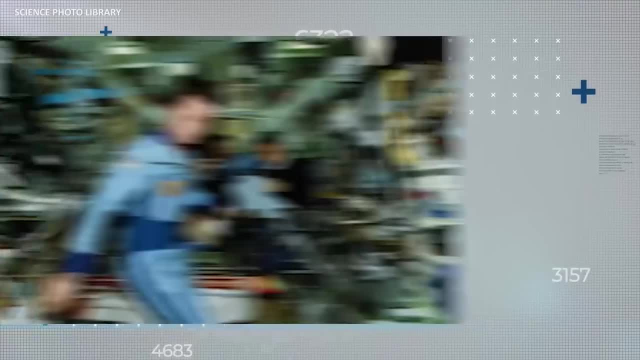 older space stations' orbital facilities On the now-defunct Russian space station Mir. a power failure once forced cosmonauts to defecate directly into emergency plastic bags until a repair could be made. Morale is said to have suffered badly. 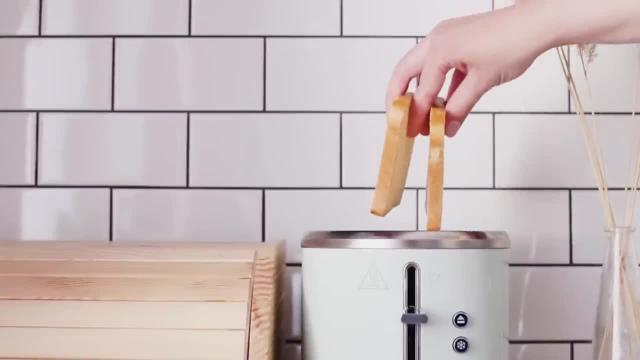 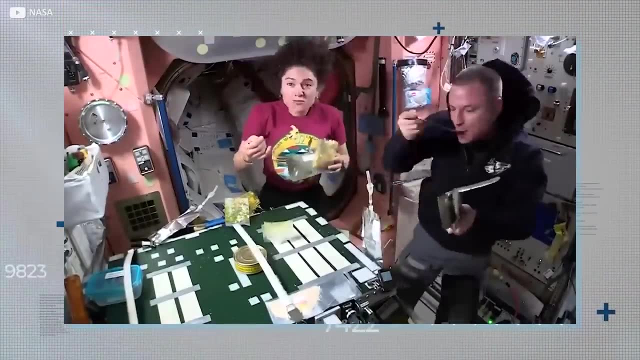 Anyway, let's go to breakfast. Toast is definitely a no-no on the space station, as are sandwiches, because crumbs are a disaster in zero-gravity environments. Not only are they messy, but if left to float away checked, they get lodged in tiny crevices and encourage the growth of fungus. 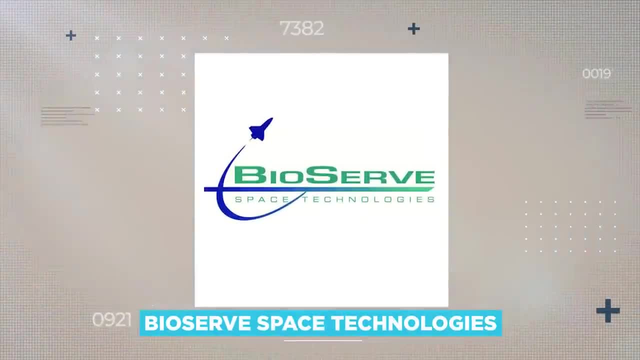 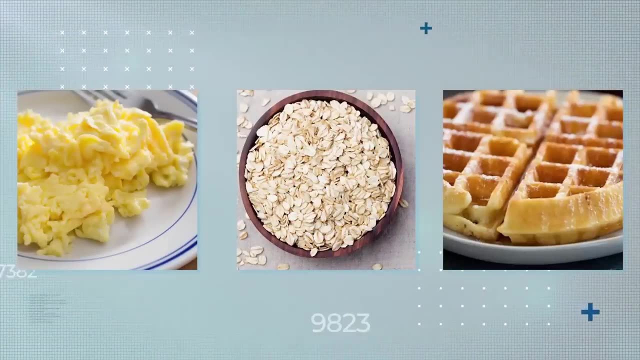 There are no conventional fridges, although a company called BioServe Space Technologies is trialing a substitute aboard right now, But there's plenty to eat nonetheless, like scrambled egg, oatmeal or waffles. True, much of it is dehydrated, brought to life with 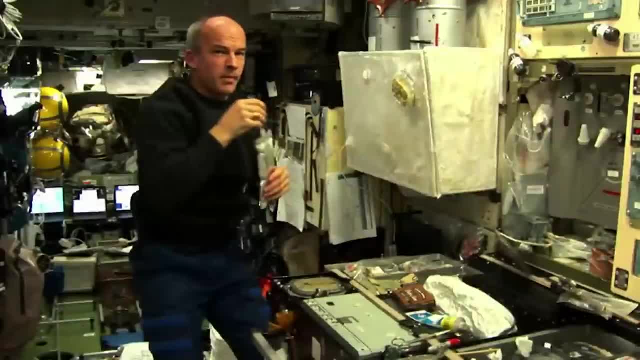 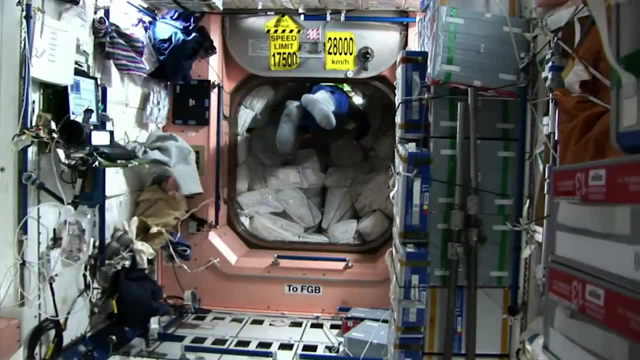 warm water, but there's also lemonade, coffee or tea, so long as you don't mind drinking through a straw, of course- After breakfast, part of a rigorously planned diet that's carefully monitored by nutritionists. it's time for a crew call to mission control. 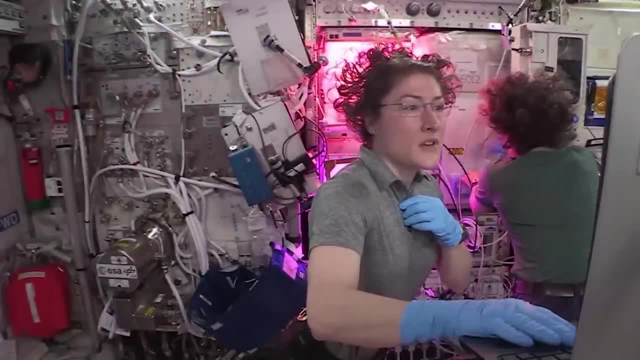 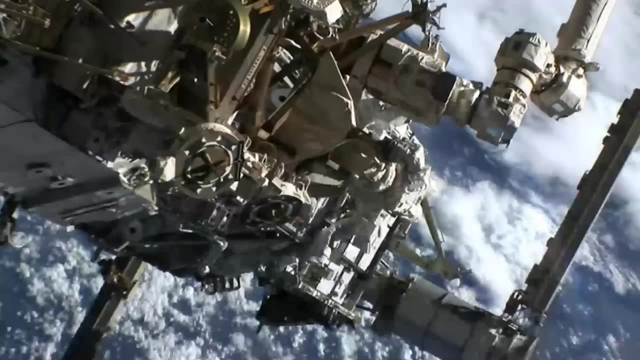 to go over the plan for the day. Nearly every single task on the ISS is carefully scripted, and astronauts have their activities planned in step-by-step fashion down to the finest detail. Some of the most important duties involve maintenance, both preventative tasks. 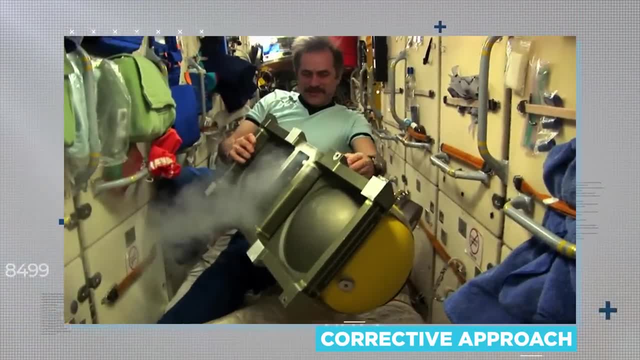 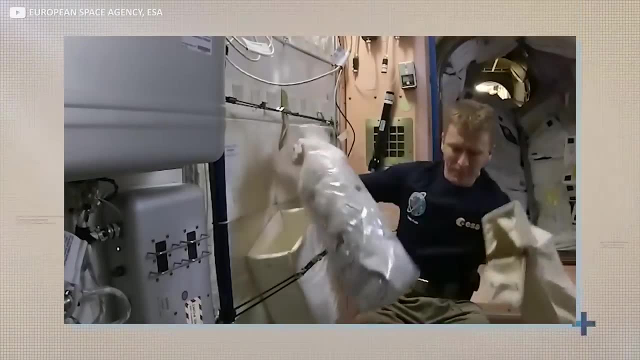 carried out before things go wrong and the corrective approach once something's actually broken. Cleaning filters is important, as is the disinfection of surfaces, updating computer software and even taking out the trash which usually goes into the Russia-launched Progress service vehicle. On occasion, the crew's maintenance. 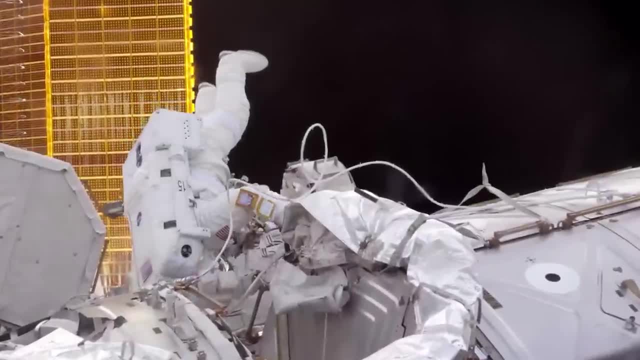 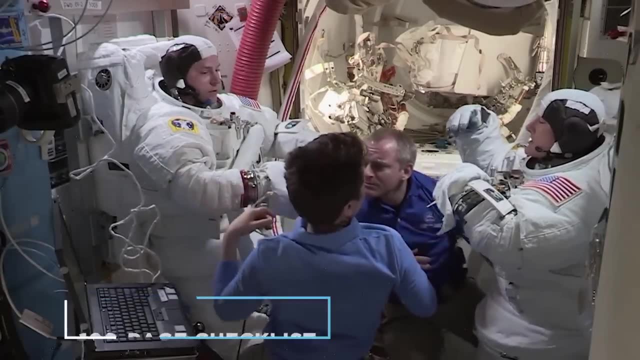 duties will require a spacewalk. This can be for jobs as apparently mundane as changing batteries on the exterior of the station but still necessitate four hours just to suit up and a 100-page checklist to run through. In case you're wondering, yes, there's a diaper in there. 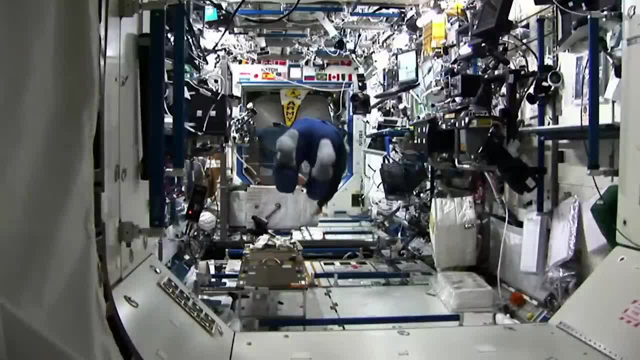 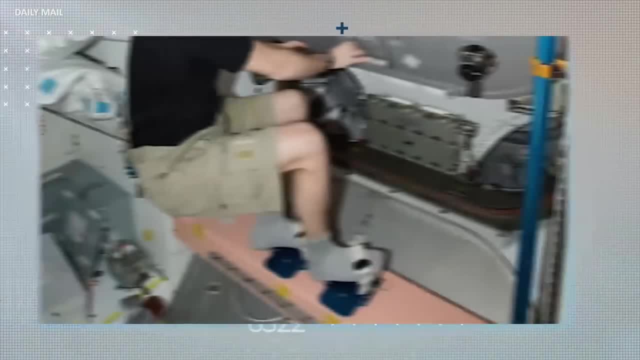 Typically, the crew move through the interior of the ISS using an array of handrails which are situated at intervals on every surface. It's said that during extended missions, astronauts' calluses vanish from the base of their feet but reappear on the top. 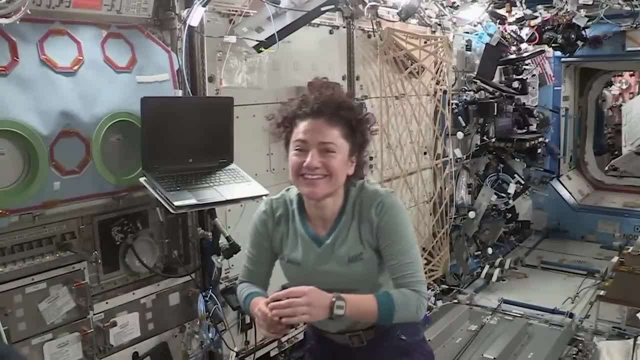 because this is suddenly a vacuum. The crew then move through the interior of the ISS using an array of handrails. This is a very crucial body part for keeping them upright and steady. As well as those handrails, surfaces in the ISS are usually adorned with strips of velcro. 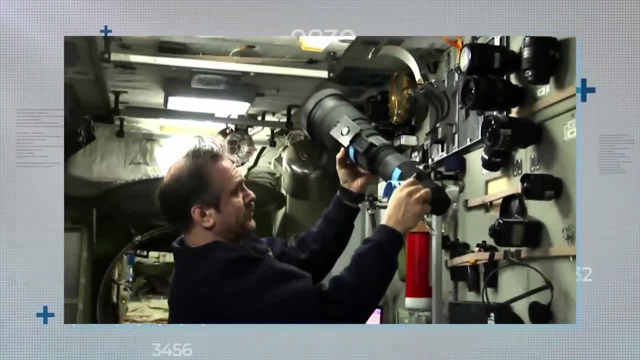 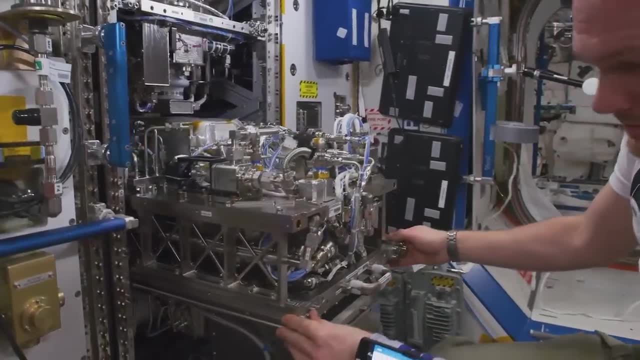 This is to help stop hand-held tools, pens and other items from drifting away and getting lost, sometimes for frustratingly long periods After a solid morning of work, often in solitary roles, but sometimes teaming up with colleagues across the Russian-English language divide. 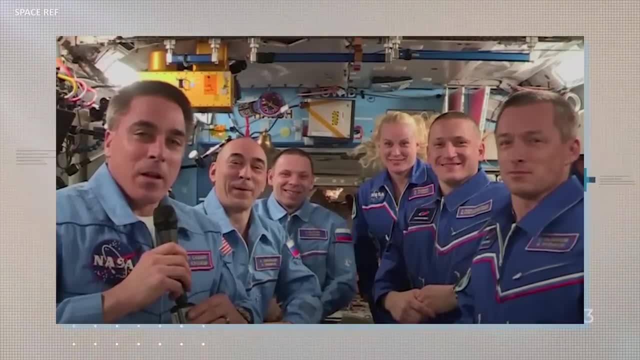 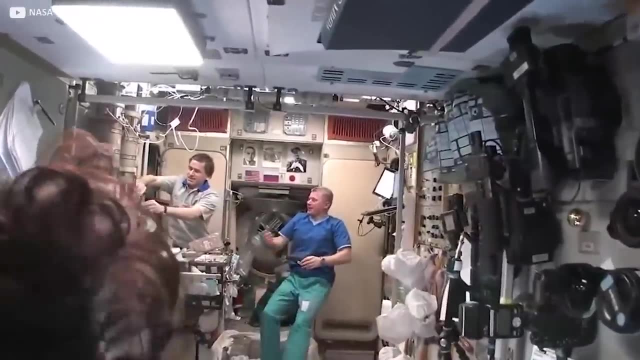 using a dialect astronauts affectionately refer to as Runglish, it's time for lunch. While the days of the week make even less sense than the days of the week and the difference between night and day in space, the ISS crews still maintain a distinction. 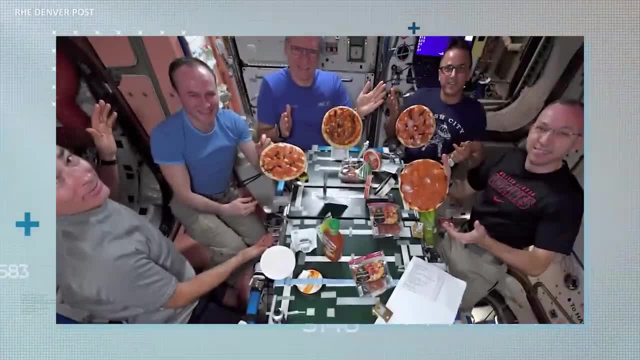 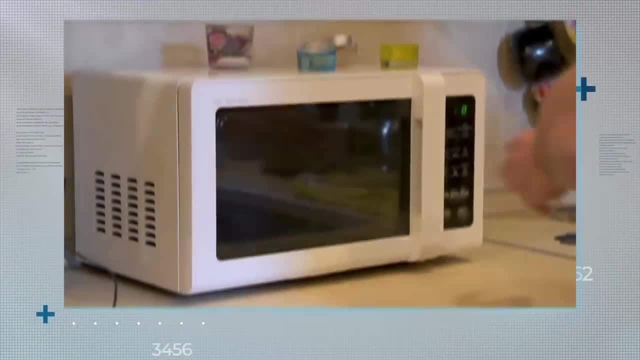 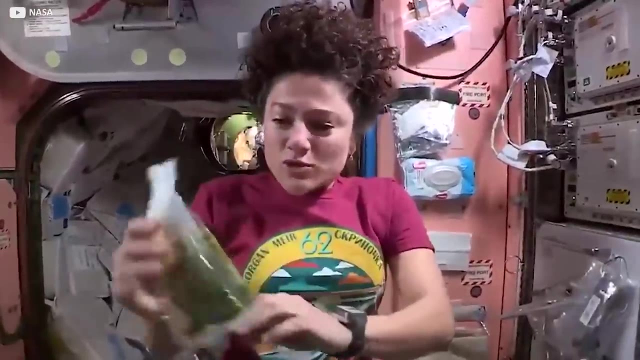 between weekdays and weekends and share a ritual meal together as a team on Sunday. Weightlessness creates issues for everything aboard the ISS, and cooking is no exception. Convection, the heating principle on which most Earth-based ovens run, doesn't work in orbit. Hence most meals are prepared from dehydrated ingredients and hot water. 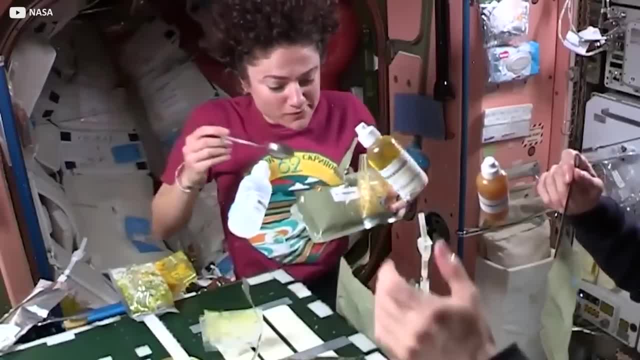 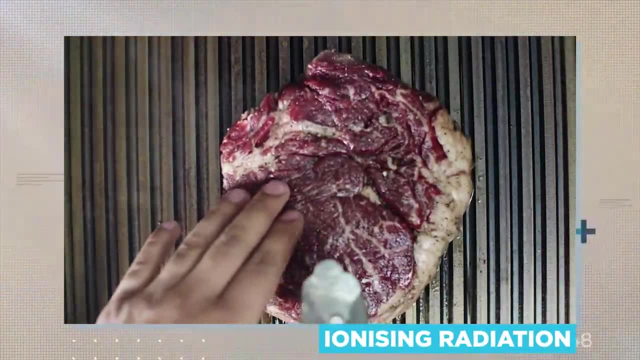 This is also to prevent fungus from taking hold amid moist stored foodstuffs. Some food items, beefsteak for instance, come pre-sterilized with ionizing radiation, which helps prevent spoilage. Condiments like ketchup, mustard or hot chili are all available to spice things up. 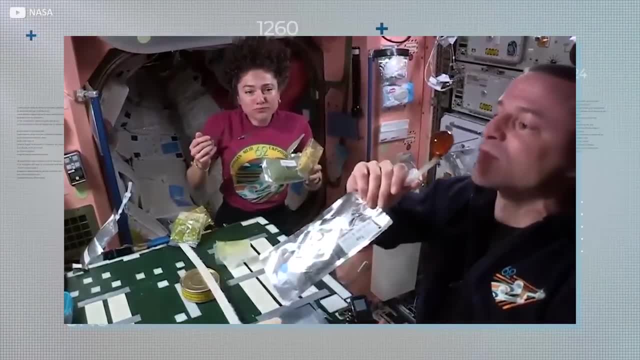 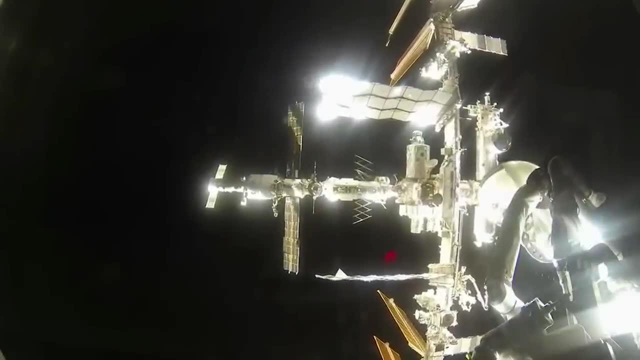 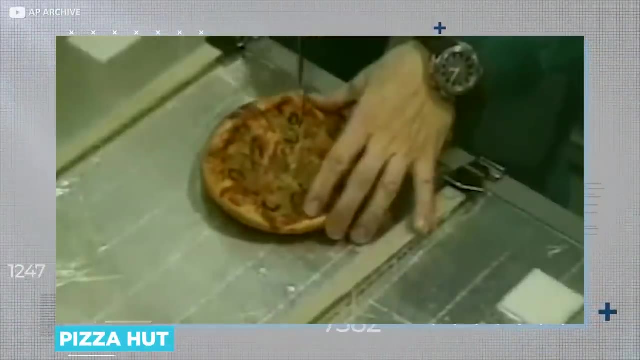 as are salt and pepper, albeit in liquid form, so the granules don't drift away and cause havoc with station operations. Deliveries of fresh food, such as fruit, happen periodically throughout the year. Takeaways aren't really an option, except for back in 2001 when Pizza Hut memorably sent a family-sized salami pizza on a Russian rocket. 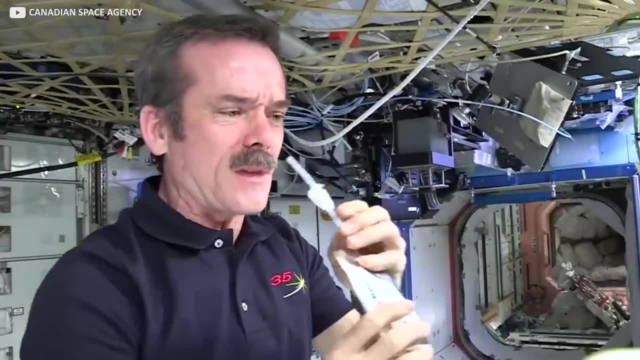 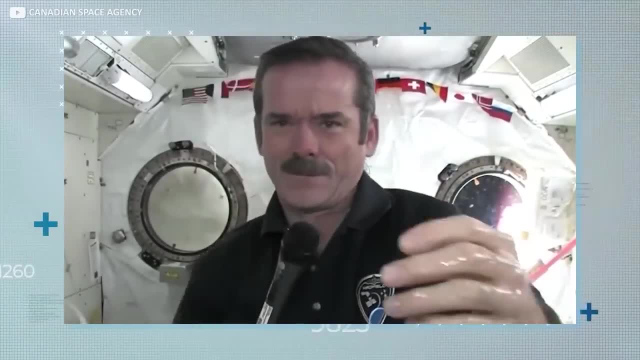 as part of a million-dollar market. Mission Control is keenly aware of the importance of fresh supplies to the morale of the hard-working ISS crew After washing their hands with disinfectant wipes- because, remember, there's no sink, it's straight back to work. The main mission for the ISS team is to conduct. 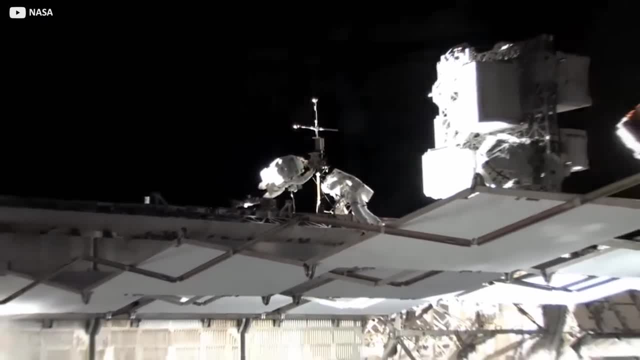 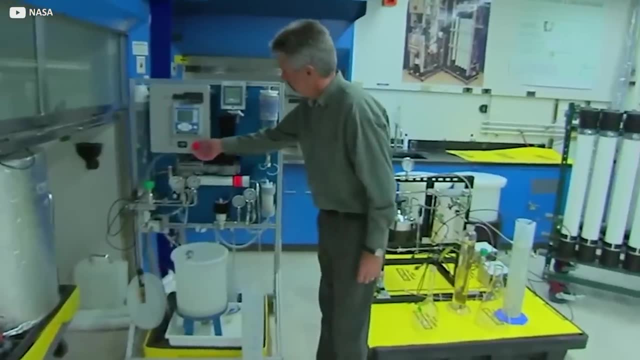 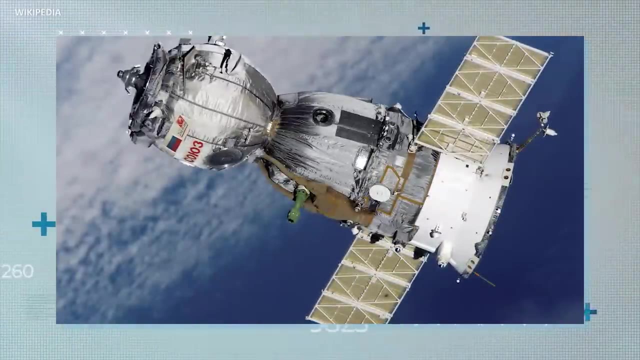 scientific experiments and further mankind's understanding of life in space. So the most important and exciting work they'll do is essentially in the role of lab technicians, guided in their actions by scientists on the ground. And the ISS is positively bristling with labs. Russia has two mini-research modules. The US lab is called Destiny. 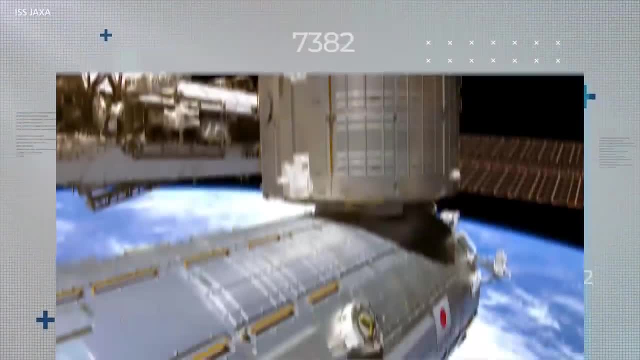 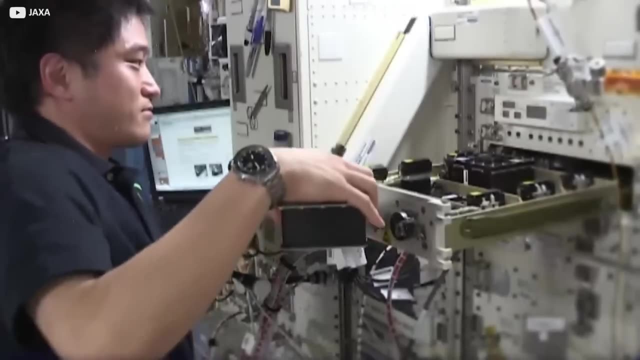 Columbus is run by the European Space Agency. The most recent lab is Japan's KAIBO, which includes a special platform allowing experiments to take place outside the station. Just some of the questions being explored concern the effects of low gravity on living cells. 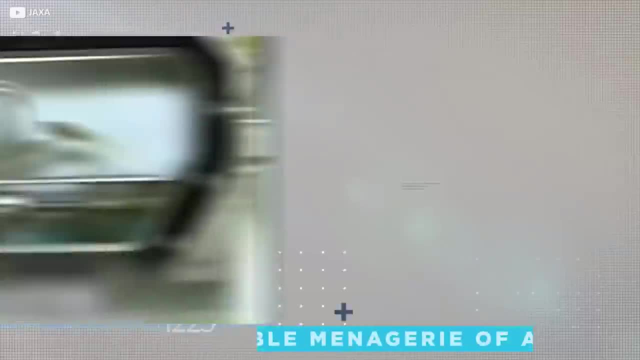 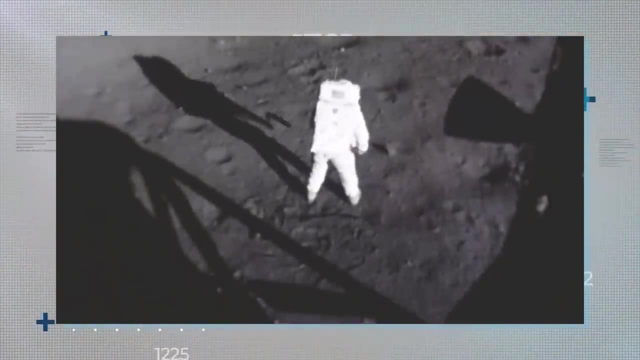 artificial materials and even miniature explosions. A veritable menagerie of animals, from mice to ants, to fish, to worms, often participate, but it's fair to say, the most regular experimental science is the one that's going to make the most sense. 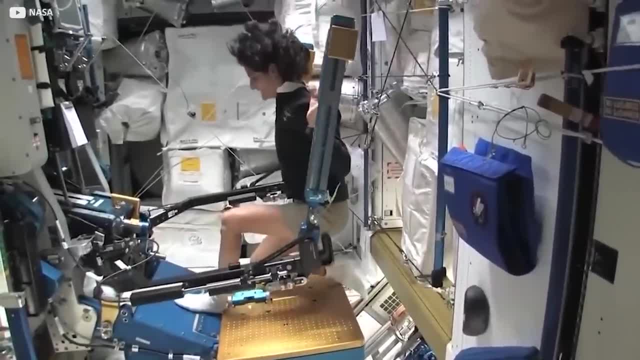 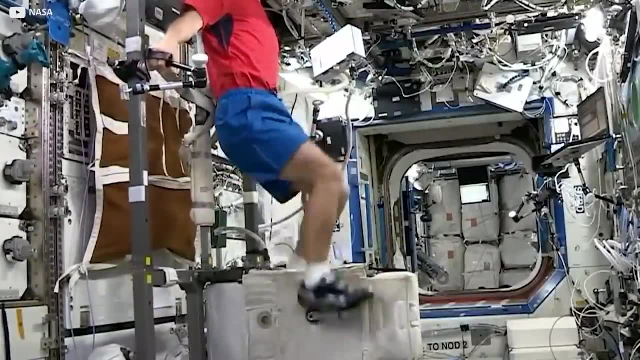 As such, they need to stay in good shape. so when all that scientific work is done, it's time to work out. Each crew member is required, as part of their duties, to work out for at least two, and sometimes more hours every day. Partly this is because 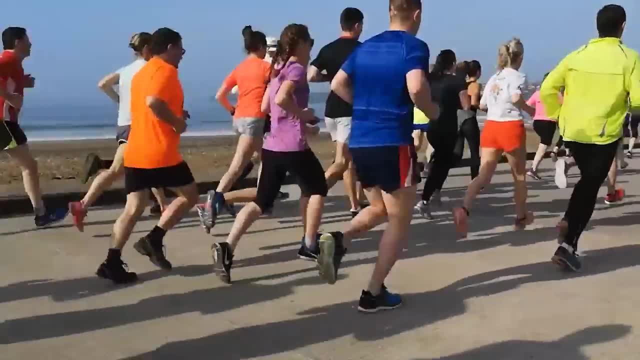 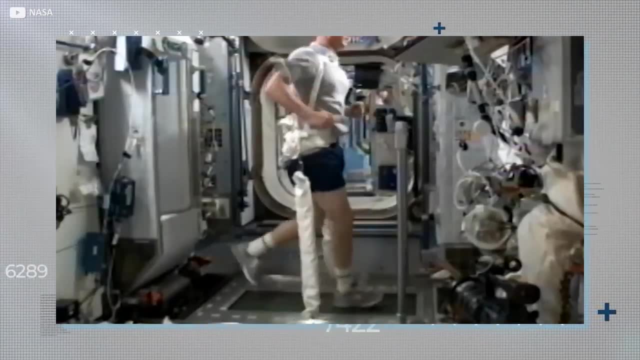 gravity on Earth naturally keeps human beings' bones and muscles in good condition, as they are constantly working to keep us upright. But in space muscles atrophy and bones grow brittle unless constantly worked. Astronauts also work out to combat the dreaded space snuffles. 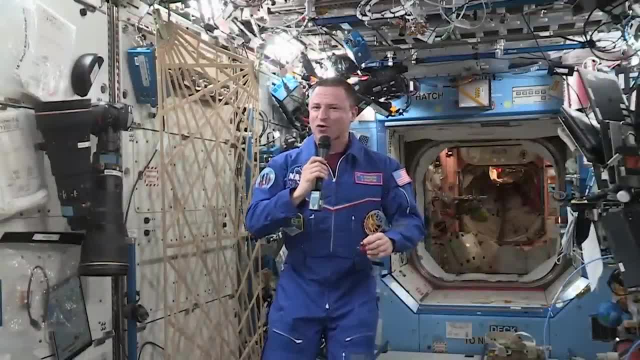 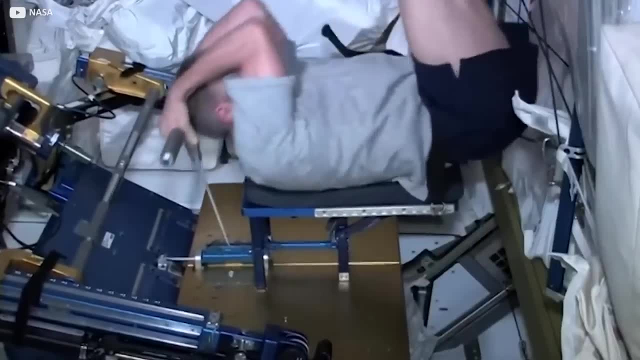 An unlovely condition where bodily fluids no longer lugged downward by gravity, accumulate in the head. In order to stay trim and clear-minded, astronauts make use of three main pieces of gym equipment specially designed and calibrated for life. on board There's an. 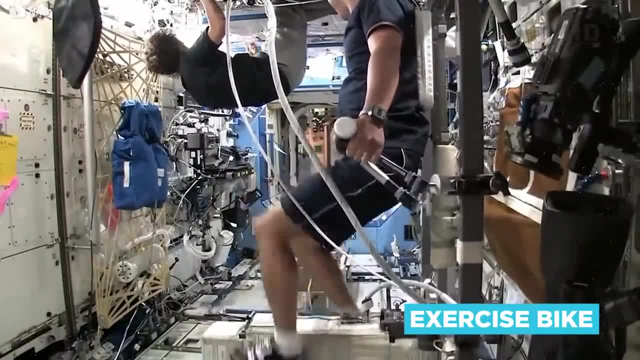 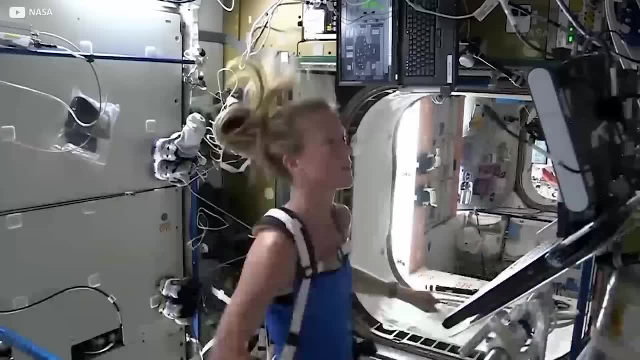 exercise bike which doesn't have a seat because you don't need one in zero gravity. There's also a treadmill onto which crew are secured with bungee straps. It has a clever vibration isolation system built in, so astronauts' heavy footfall can't disturb the delicate science going on. 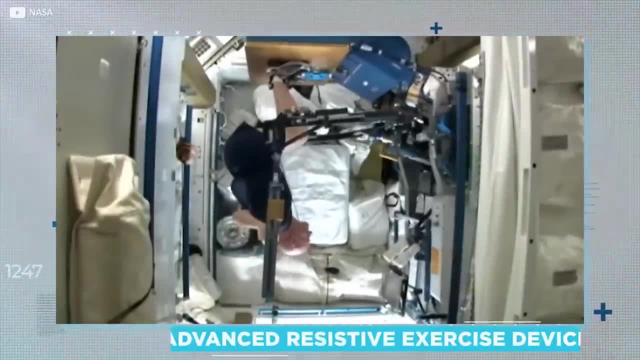 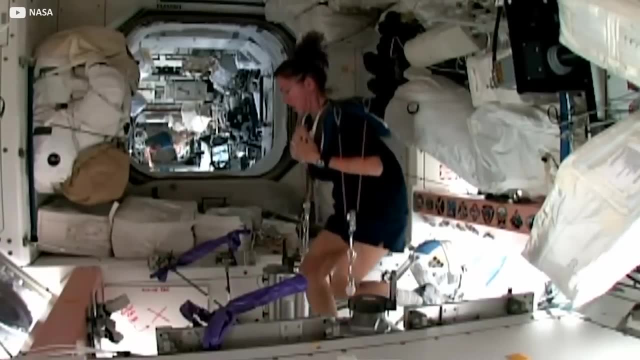 around them. The third main piece of workout equipment is the so-called Advanced Resistive Exercise Device, or ARED, The most recent addition to the ISS onboard gym. ARED uses clever vacuum-sealed cylinders to mimic resistance. up to 600 pounds as an alternative to lifting. 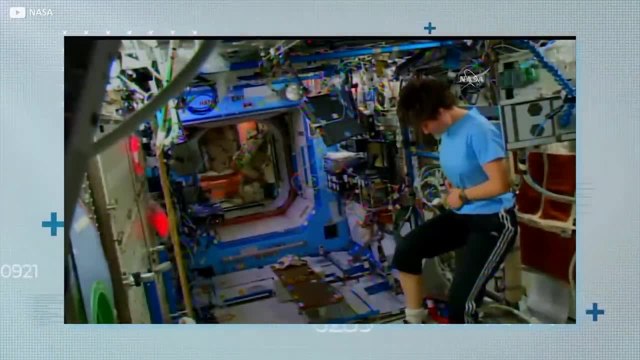 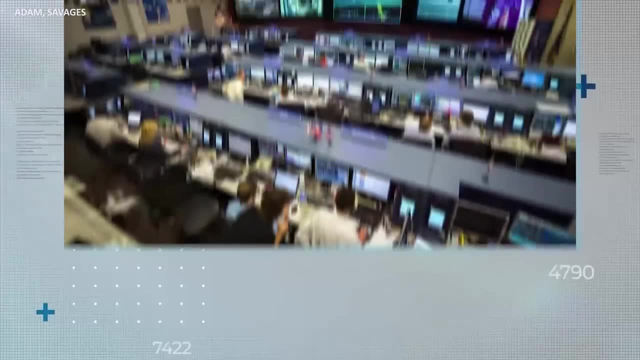 heavy weights. If you're wondering how astronauts cope with the sheer tedium of pumping iron for two hours every day, while teams on the ground monitor their vital signs and provide coaching, don't worry, There are screens for watching movies and even scope to get competitive In 2012,. a NASA 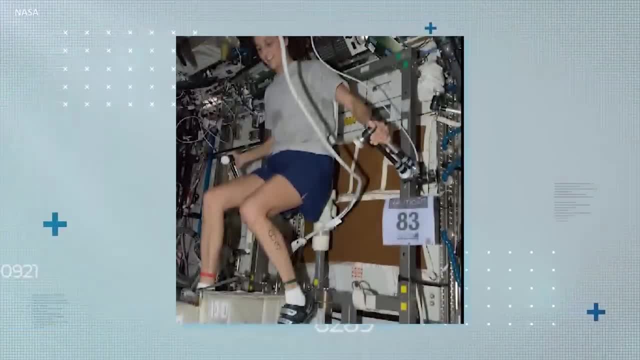 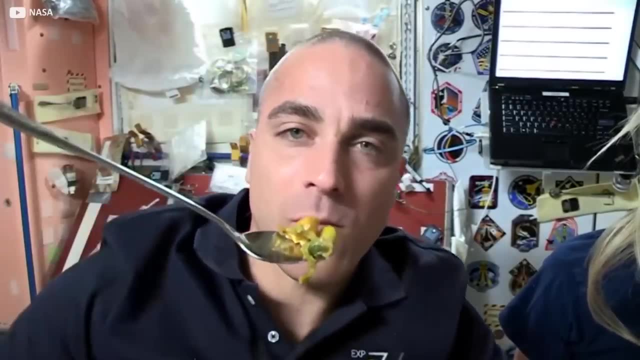 named Sunita Williams, competed in the Malibu Triathlon using ARED as a makeshift swimming simulator. What's your excuse After an evening meal which can sadly taste a little bland, as aroma doesn't really work in low gravity and blood surges to the sinuses thanks to those space?